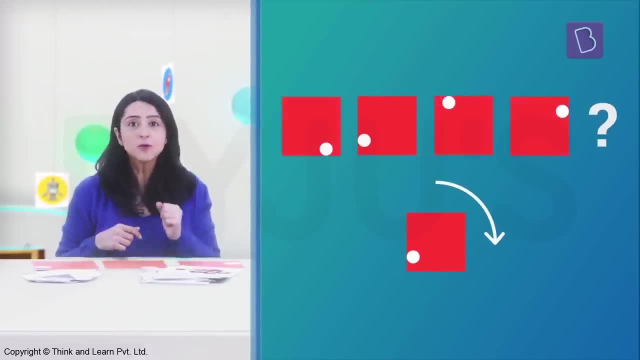 That's good news. If you look at it, I gave a one-fourth or a quarter turn to this shape in the clockwise direction. Now why do I call it a one-fourth turn? This is because if I turn it like this three more times, I finish one full turn. 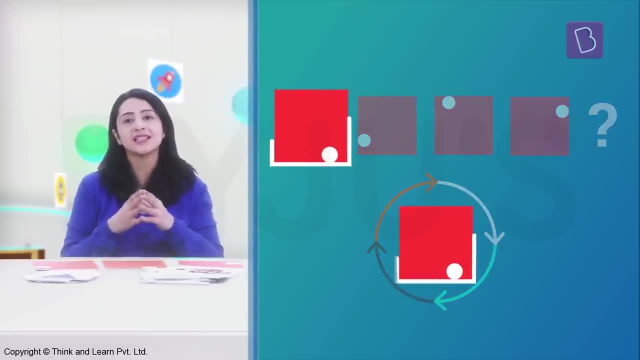 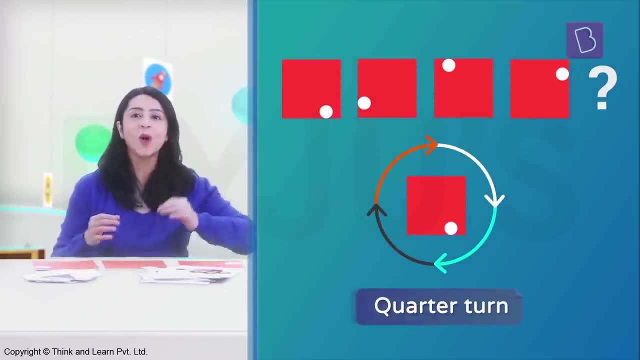 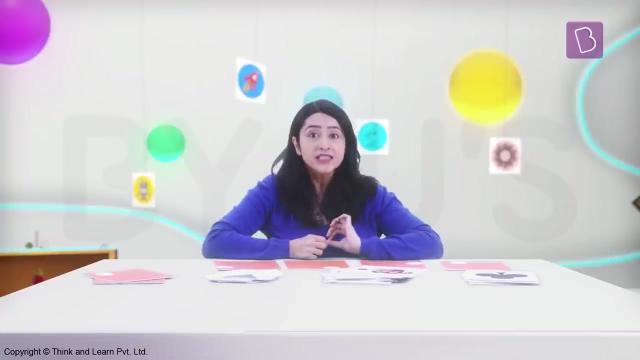 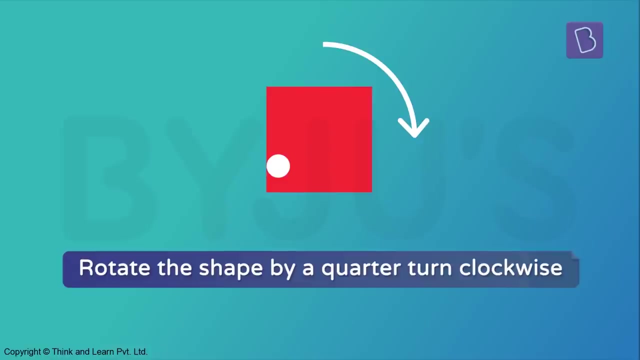 and the picture comes Back to where I started. For this reason, we can also call this a quarter turn. This is good, So let's note this down. The possible rule for this pattern is rotate the shape by a quarter turn, clockwise. All right, let's do that again on the second piece. 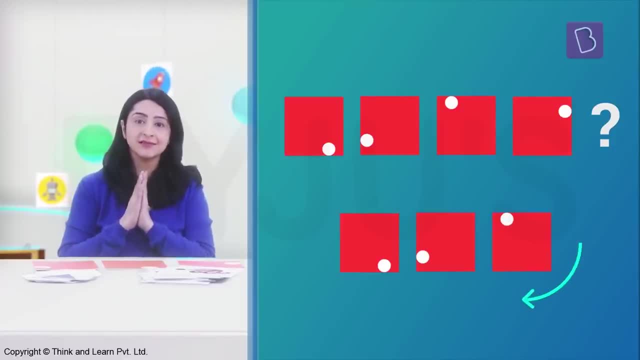 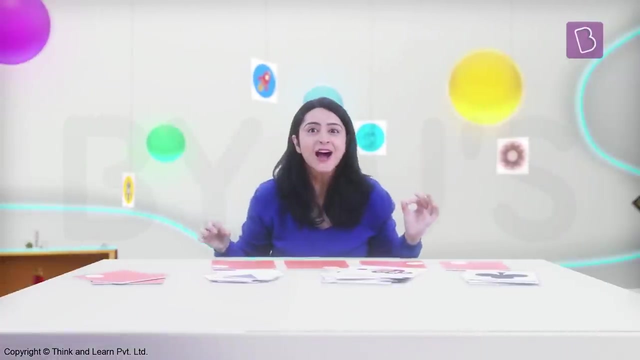 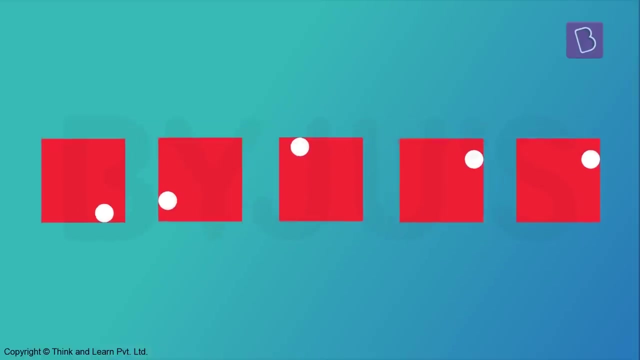 And we give it a quarter turn. Ah, the third piece matches. If I continue to do it for the remaining shapes they match exactly. And there you go. We found the rule for this pattern. Now, to get the next shape in the pattern, I just replicate the fourth piece and give it a quarter of a turn clockwise. 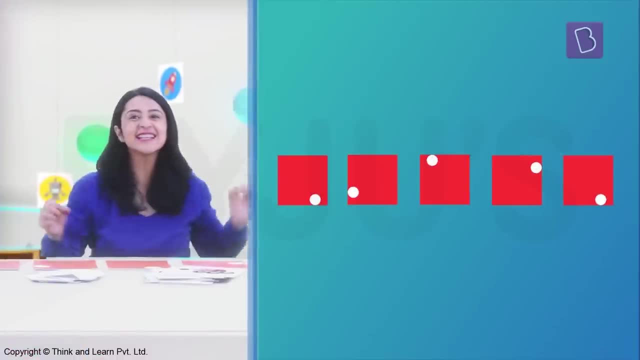 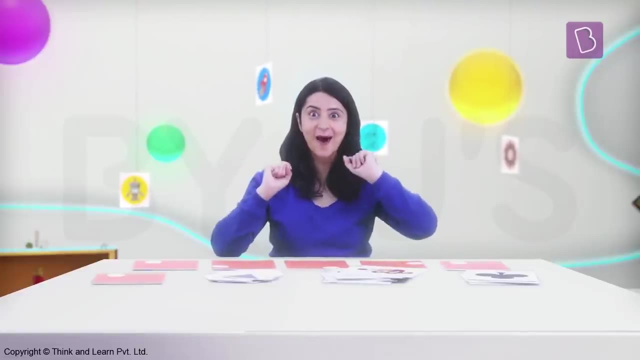 Like this, And that is the missing piece. Yes, Thanks to you, this puzzle is over. Now, with the same spirit, let's learn more about patterns like these. This quarter turn rule is one rule to solve pattern puzzles, But is that the only rule? 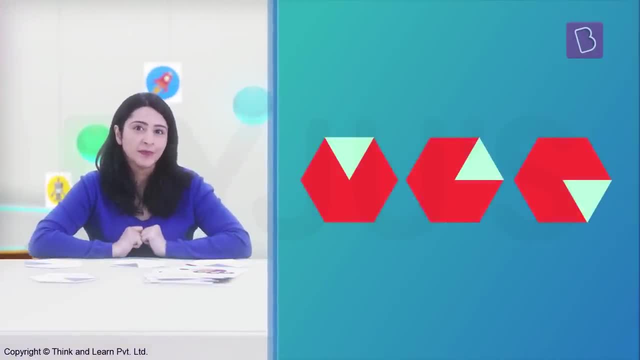 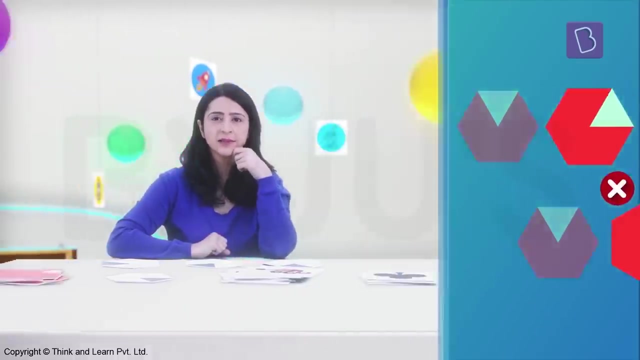 Ah, let's take this, This puzzle, over here Now. here also, we need to find the next piece. What if I turn the quarter, turn clockwise rule here? Ah, it's not working, It's all right, These things happen. 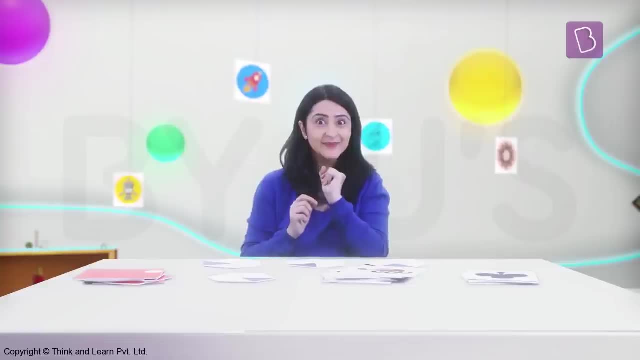 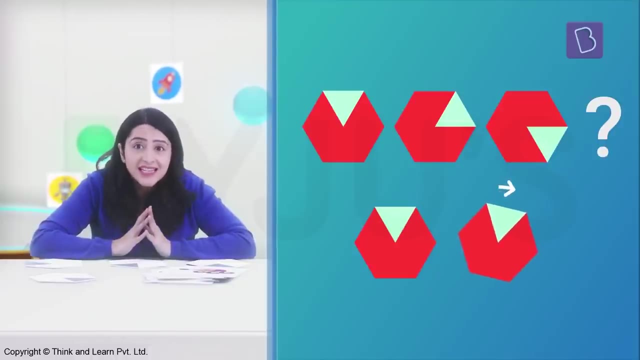 Sometimes you don't get the answer in the first try, right, So let's try it again. I take the first piece of the pattern and rotate it Till it looks exactly like the second piece, Like this. Now, if I try this, turn for all the other pieces. this works. 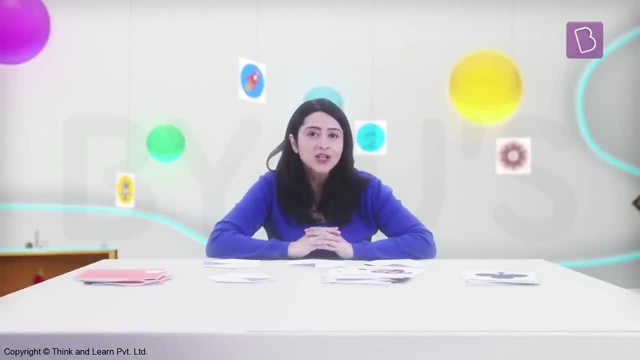 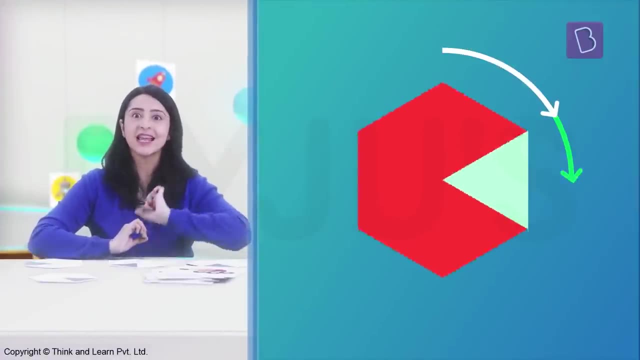 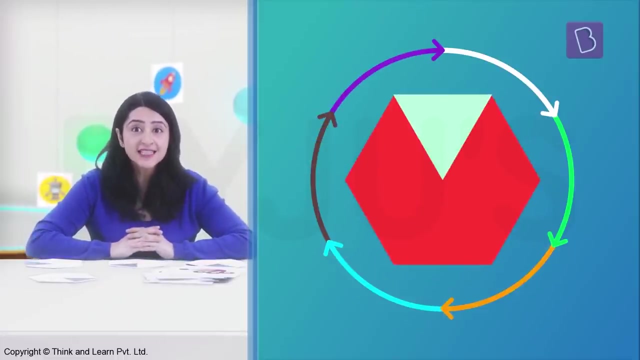 Now, this turn is special. It's not a quarter turn, So to find the name of this turn, let's try to give this piece the same turn again and again. You'll notice That after six turns the piece comes back to the same position we started with. 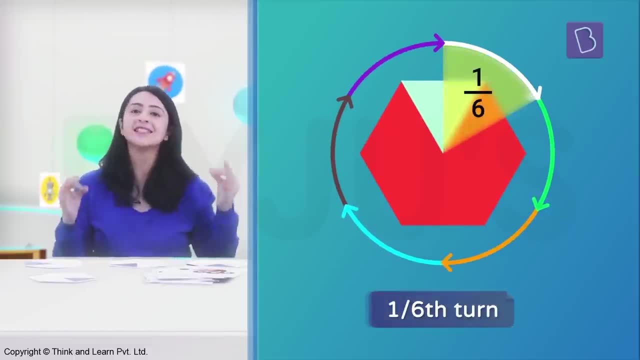 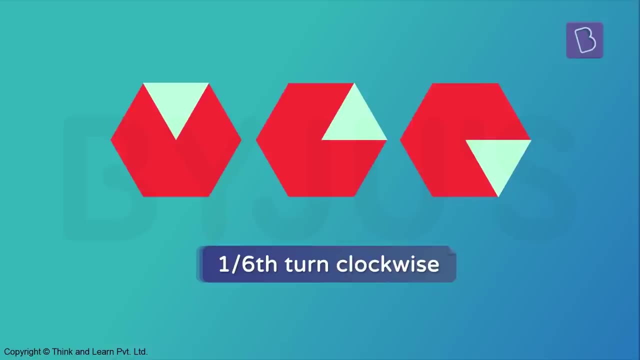 So this turn is called a one-sixth turn. So the rule for this pattern is one-sixth turn, clockwise. So if I try this rule with the third piece, I get the next piece in the puzzle Like this, And there we go. 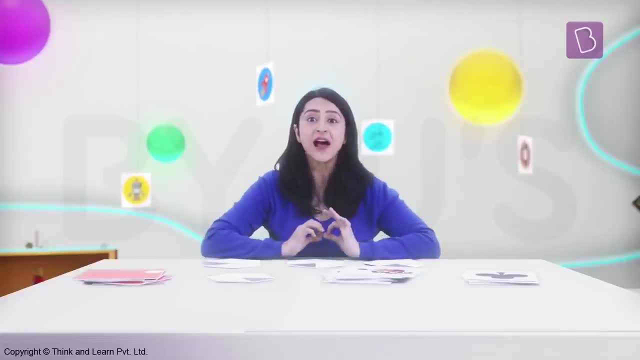 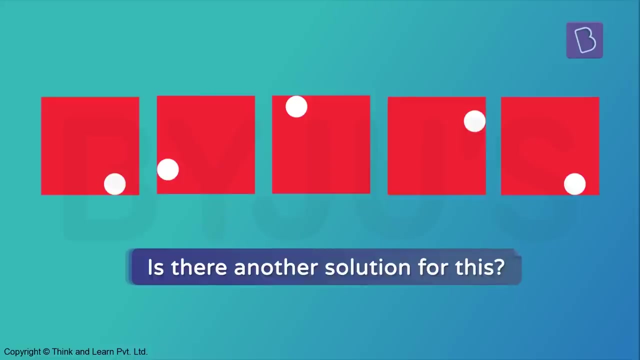 Hey, now here's a fun fact about these pattern puzzles: They have more than one correct rule. Let me go back to the first puzzle again. Tell me, is there another solution for this? Why don't you pause the video and check it out? 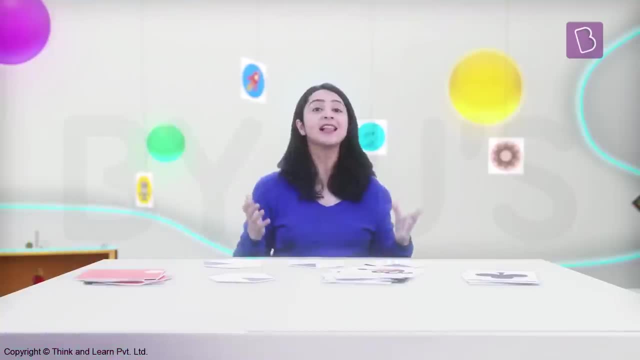 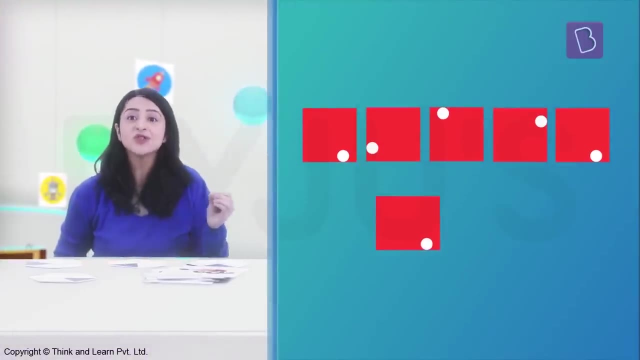 Did you find the answer? Well, I found one. Let me take the first piece, and this time I rotate it anti-clockwise. If I make a three-quarter turn, the second shape matches. If I try this for other pieces in the puzzle, this rule actually works. 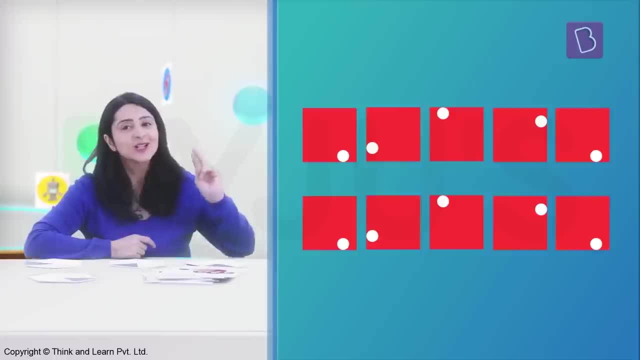 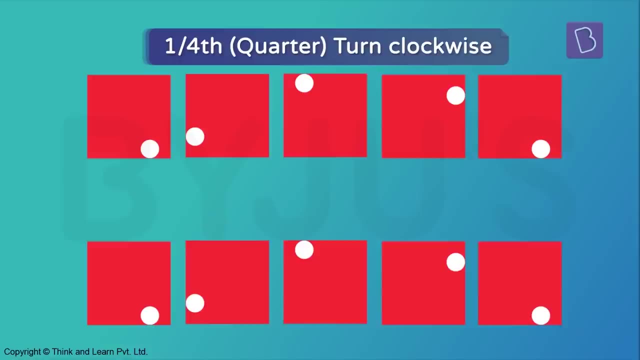 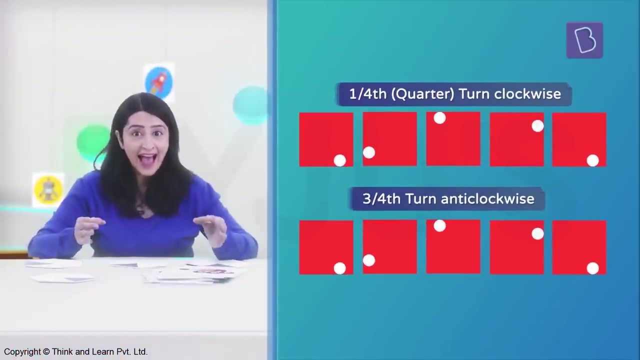 So this pattern puzzle has two rules. We rotate the pieces a quarter turn clockwise or three-quarter turn anti-clockwise. Both the rules are the same as they both give the same answer. So to solve this pattern puzzle we can use either one of them. 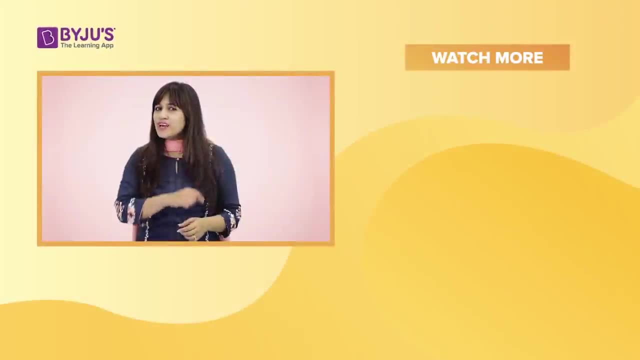 It's just a matter of convenience. If you like this video and want to watch many, many more amazing videos like these, like and subscribe to our channel now.